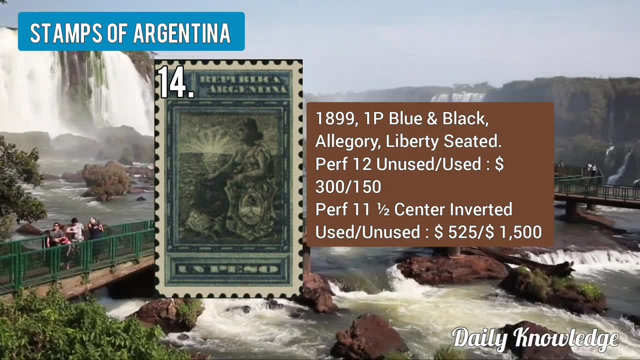 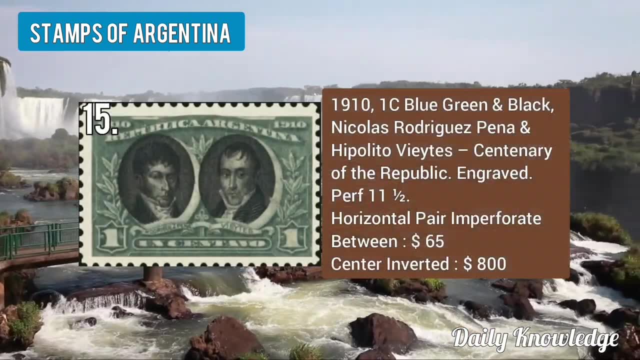 1893, 12P- black allegory, un-watermarked. 1899 1b, blue and black. allegory and liberty, seated with perforation 12.. now this one is 1910: 1c- blue, green and black. nicholas rodriguez pina and hippolyto vites. 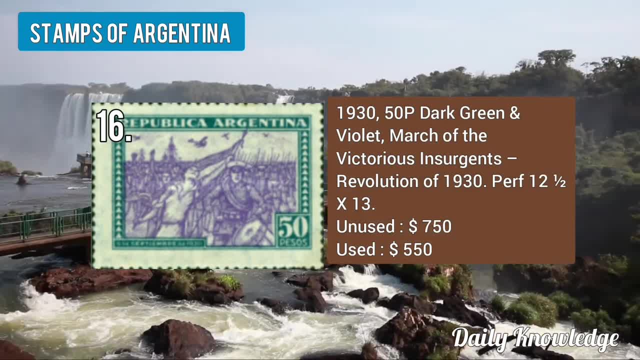 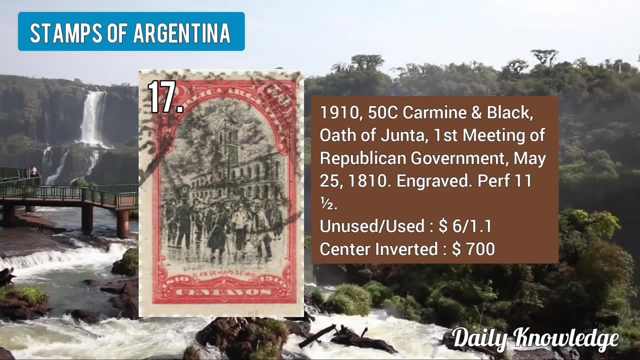 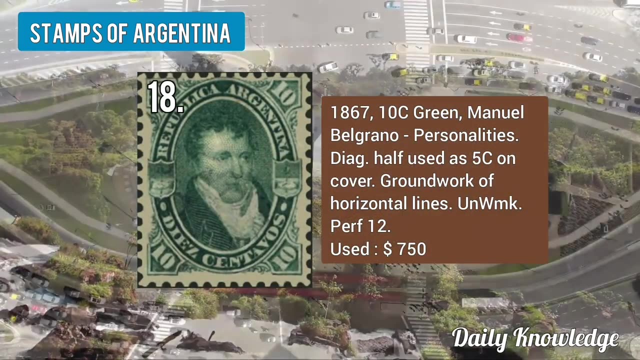 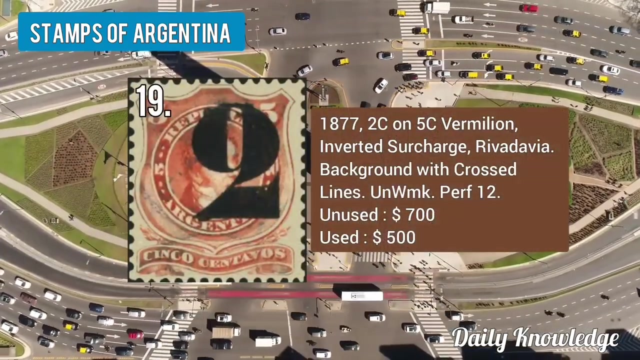 1930, 50p, dark, green and violet march of victorious insurgents. 1910, 50c, carmine and black oath of junta, first meeting of republican government. now this is 1867 10c, green manual, belgreno diagonal, half used as 5c on cover. 1877, 2c on. 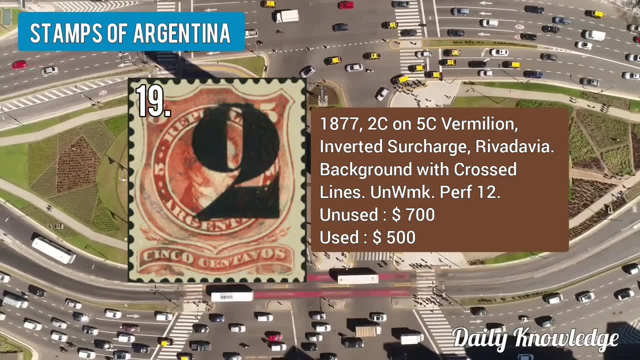 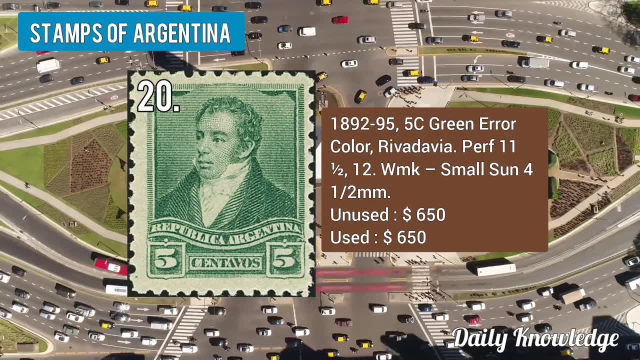 5c- vermillion inverted surcharge, river devio, background with crossed lines 1892-95. 5c- green error color river devia, with perforation 11 and a half 1910. 5p- orange and violet oath of junta made. 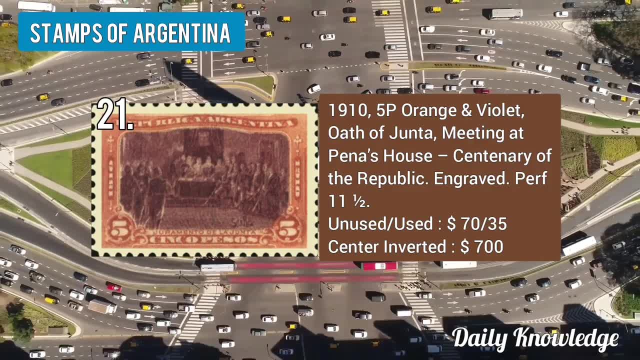 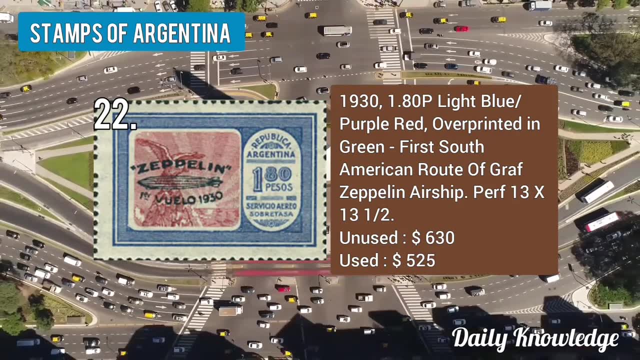 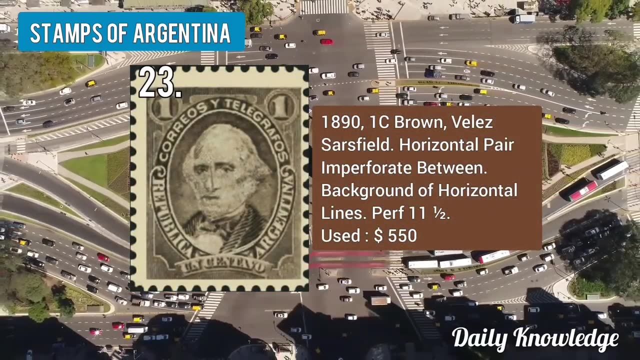 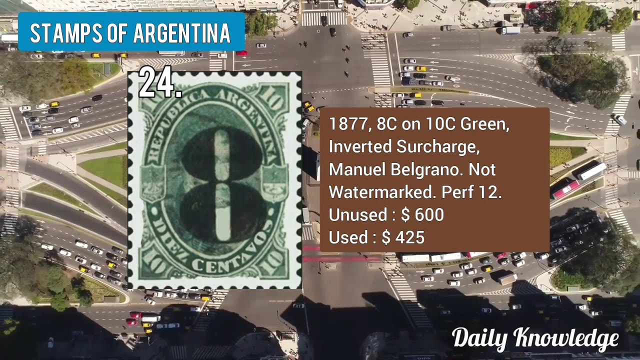 with the yellow and the green handrails meeting at Venus House. Centenary of Republic- 1931.80p. light blue, purple, red, overprinted in green. 1891c brown Baylis-Hartsfield horizontal pair, in-perforated between 1877.8c on 10c green inverted surcharge. 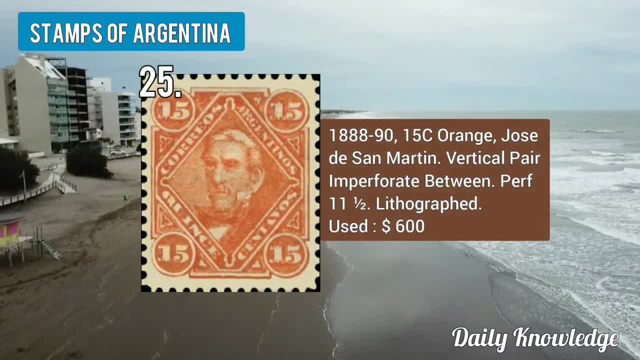 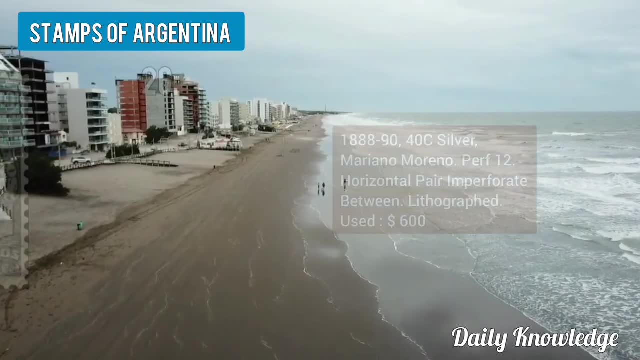 manual: Belgrano, un-watermarked with perforation, 1888-90- 15c. orange, Joss D St Martin, vertical pair in-perforated between 1888-90- 40c silver, Mariano Moreno, perforation. 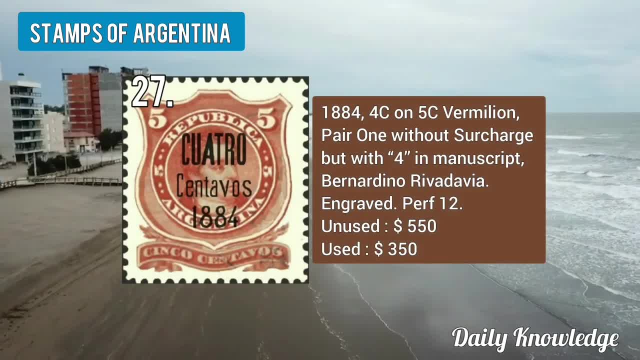 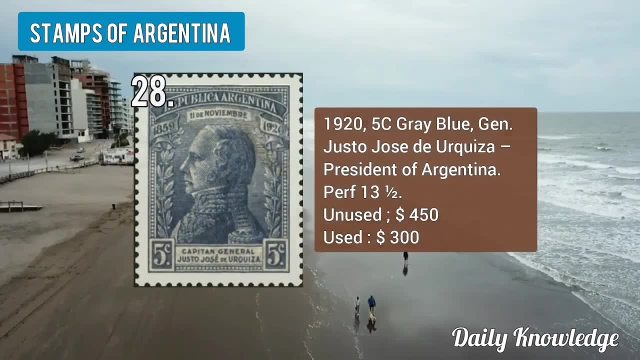 12, horizontal pair in-perforated between 1884: 4c on 5c vermilion pair 1 without surcharge but with 4 in manuscript. 1925c, grey-blue, un-watermarked, with perforation. 1888-90, 15c, orange, Joss D, St Martin vertical. 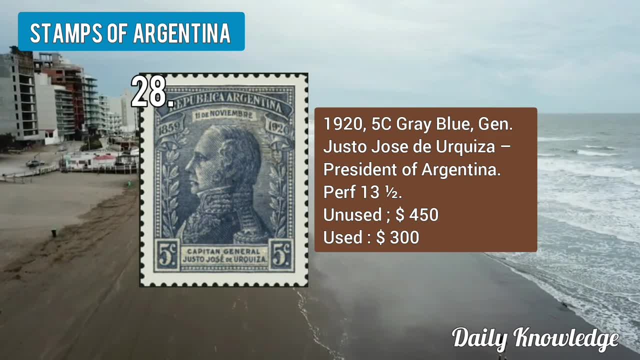 pair, in-perforated between 1888-90: 15c. silver Mariano Moreno, perforated between 1888-90- 1898-90. 20-peak green Admiral Guillermo Broun, engraved and perforated: 11.5. 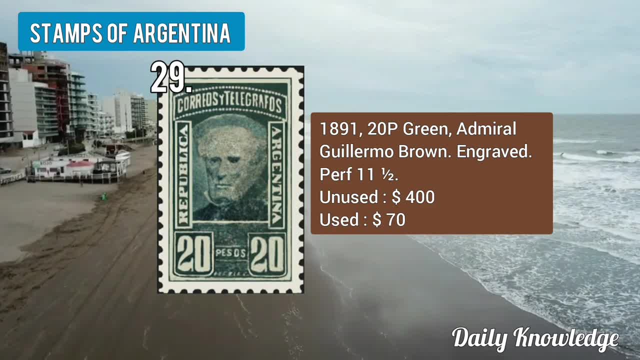 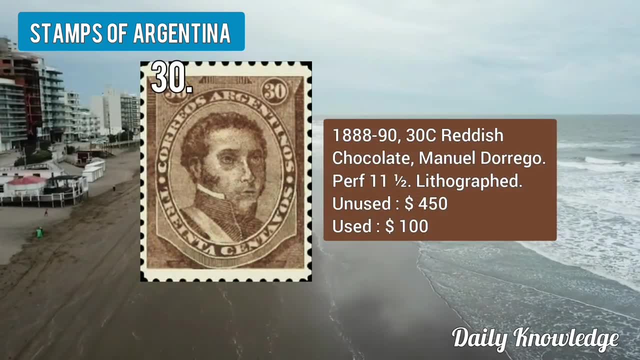 1888-90 30c reddish chocolate manual. having a red multitude of little green blue line on the one side of the pair and a circle with dark spots ruin theters adjoining them out and buttering them to the genitals. 1888-90 30c reddish chocolate manual. 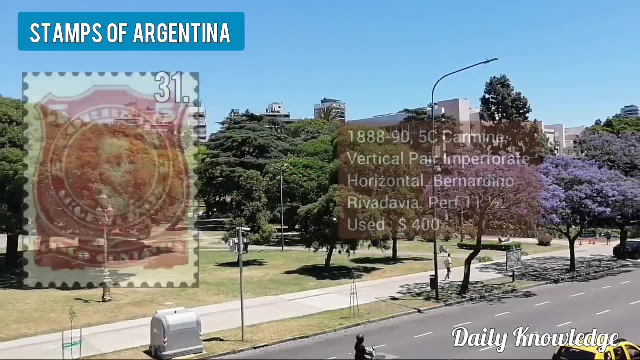 7 Dorigo, perforation 11.5 and lithographed. 1888-90- 5c. Carmine vertical. pair in-perforated horizontal with perforation 11.5, 1886-90- 30c. reddish chocolate. 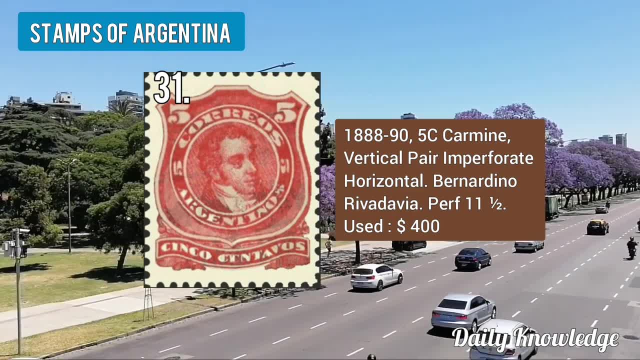 1888-90 20-green Admiralpatrick Zuschner brown, engraved and perforated- 11.5. 1888-90 30c reddish chocolate manual and lithograph warranty. 1888-90 5c- Carmine vertical pair in-perforated horizontal with perforation- 11.5. 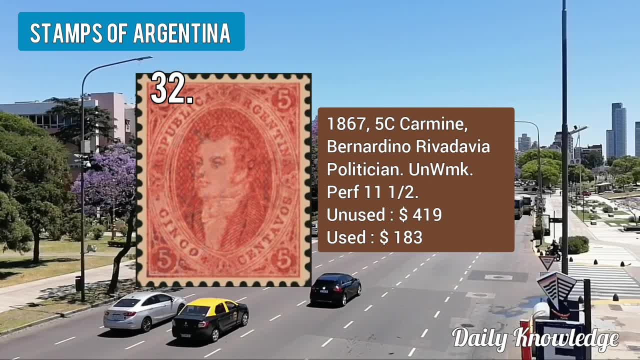 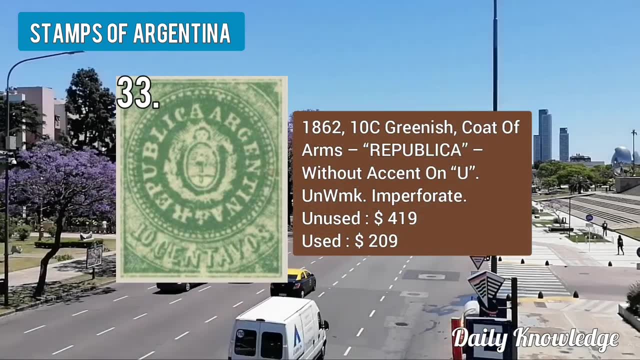 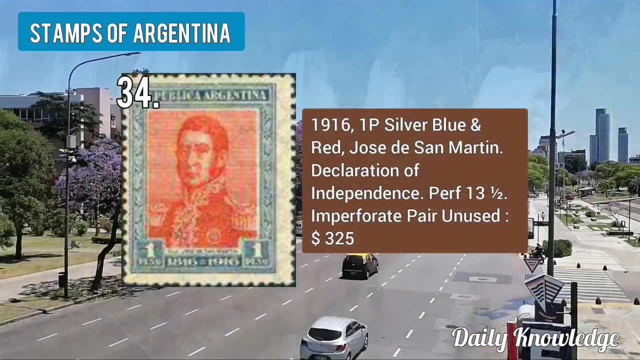 1867: 5C, Carmine, Bernardino, River Davia, un-watermarked, and perforation- 11 1⁄2. 1862: 10C- Green Coat of Arms, Republica without ascent on Jew. 1916: 1P- Silver, Blue and Red. Joseph D San Martin, Declaration of Independence and perforation- 13 1⁄2. 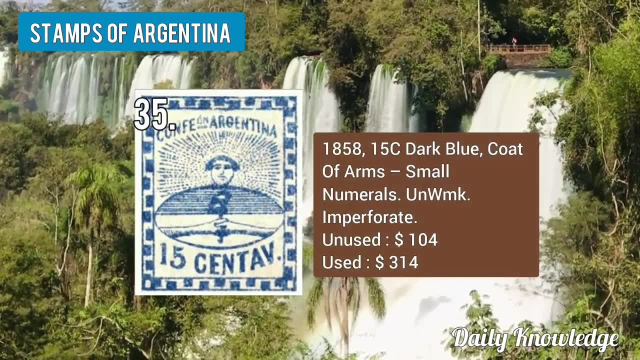 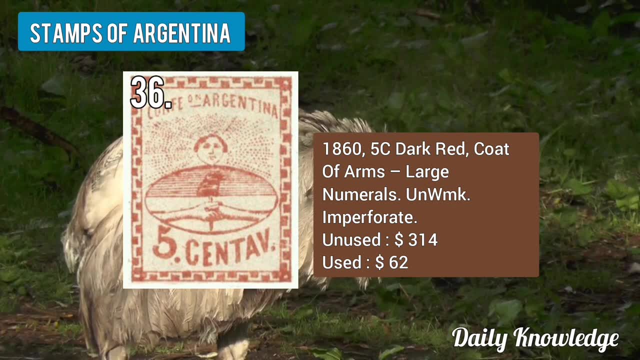 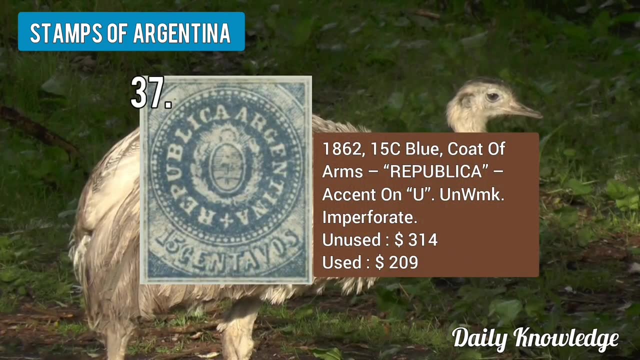 1858: 15C. Dark Blue Coat of Arms, small numerals, un-watermarked and imperforate. 1860: 5C- Dark Red Coat of Arms, large numerals, un-watermarked and imperforate. 1862: 15C Blue Coat of Arms. Republica ascent on Jew. 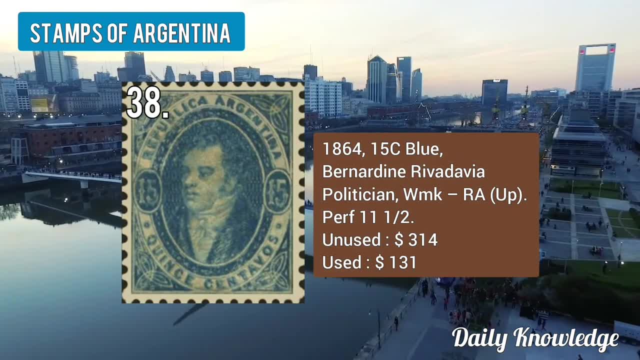 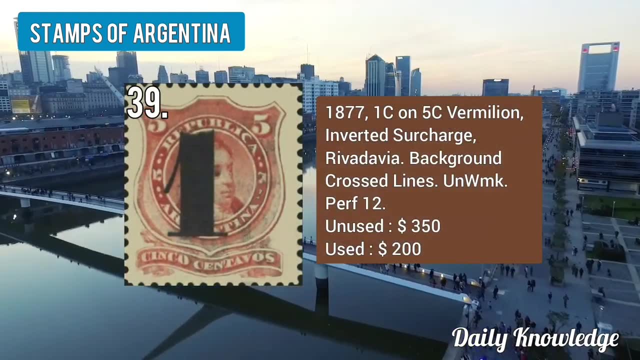 Now this is 1864, 15C Blue Bernardino River, Davia, politician, watermarked RA and perforated 11 1⁄2. Now 1877, 1C on 5C, Vermilion inverted surcharge. background of crossed lines. 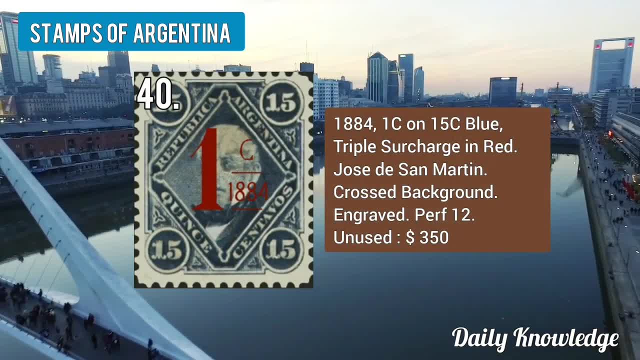 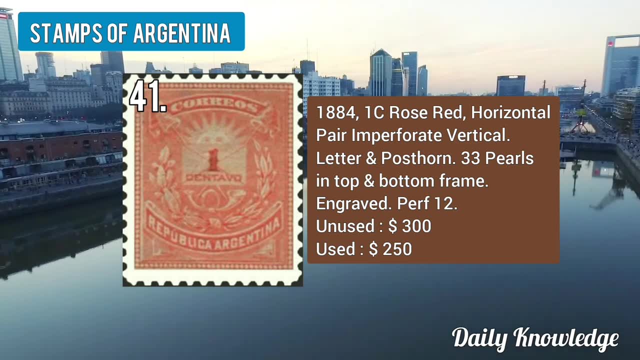 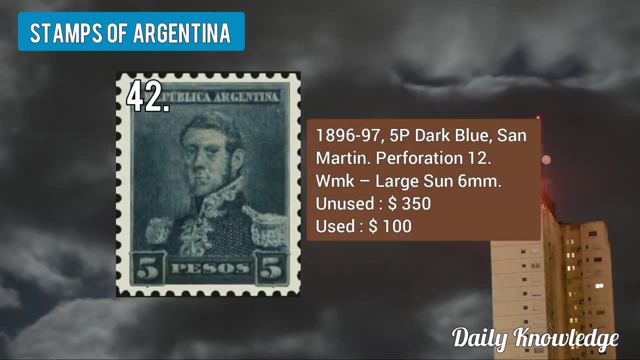 1884 1C on 15C Blue triple surcharge in red Joseph D San Martin crossed background: 1884 1C- Rose Red horizontal pair imperforate vertical later and post-form: 1896-97 5P Dark. 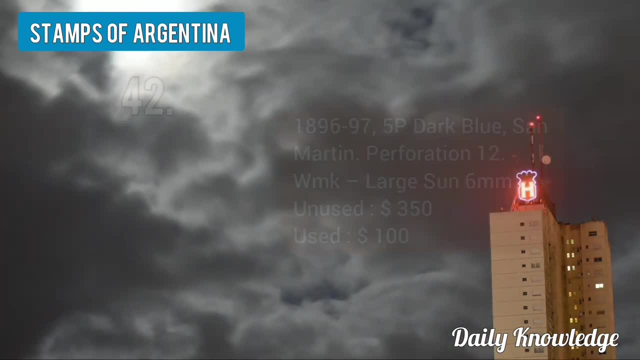 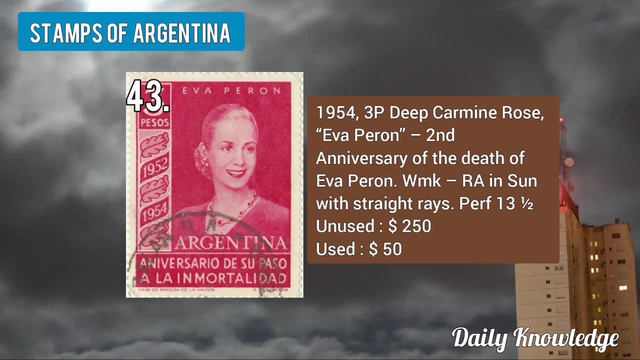 Blue Saint Martin perforation, 12: 1C and watermarked large sun. Now this is 1954. 3P- Deep Carmine Rose. Evapuron's second anniversary of the death of Evapuron- Now this is 1911. 3C- Orange, 1895. 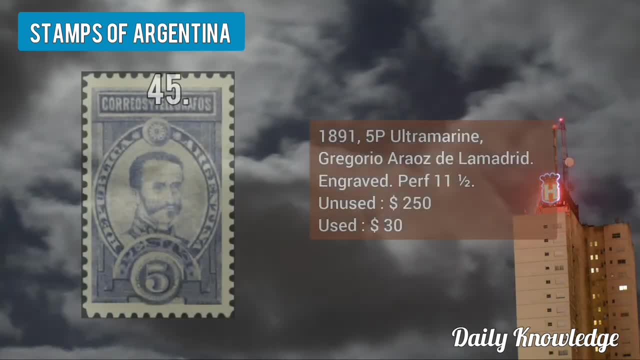 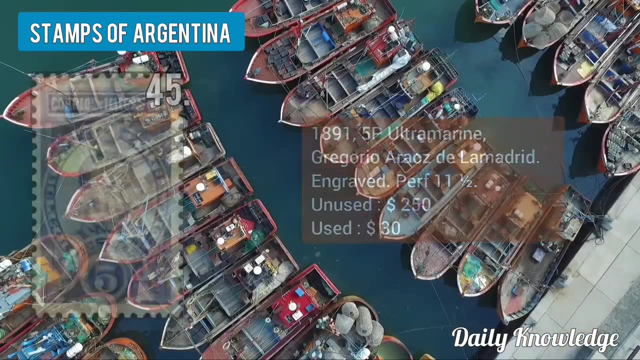 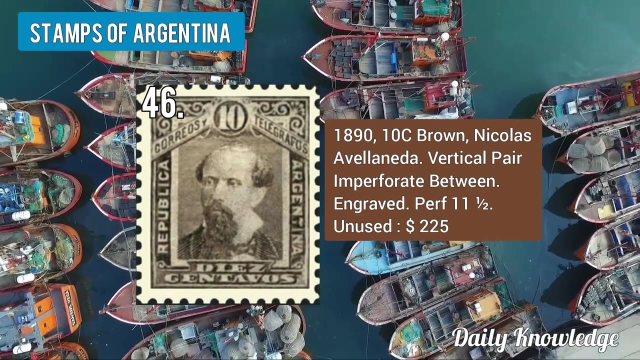 River Divya with watermarked small sun, 4.5 mm, now 1891, 5P. ultramarine, Gregorio Araoz de La Madrid. it is engraved and perforated. 11.5mm, 1890, 10C. Brown-Nicholas-Avalaneda vertical pier, in-perforated between. 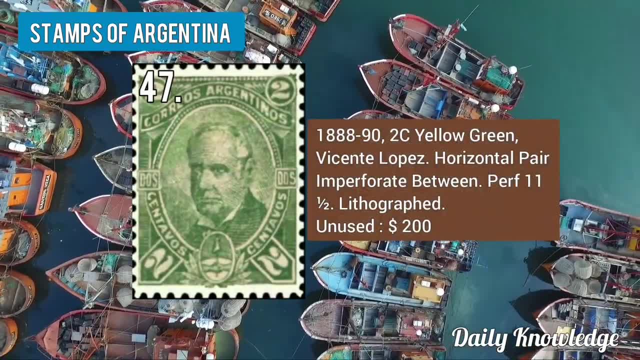 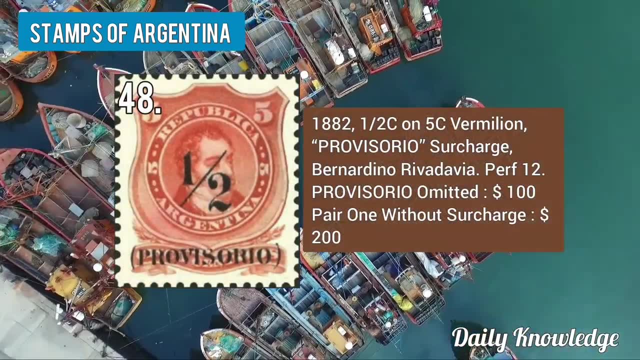 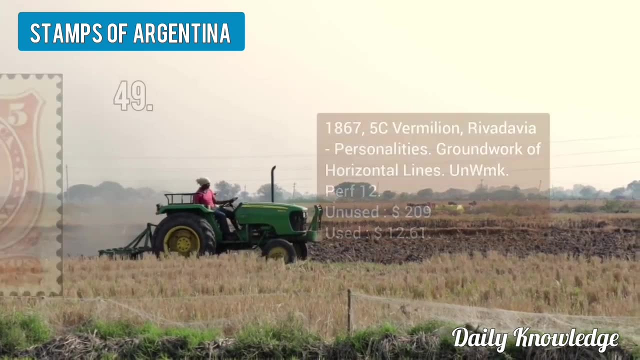 1888-90: 2C, Yellow-Green-Vicente Lopez horizontal pier in-perforated between 1882 1⁄2C on 5C Vermilion provisorio, surcharge Rivadavia, perforation 12. 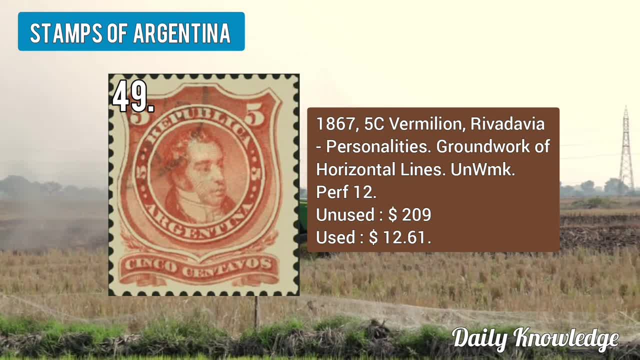 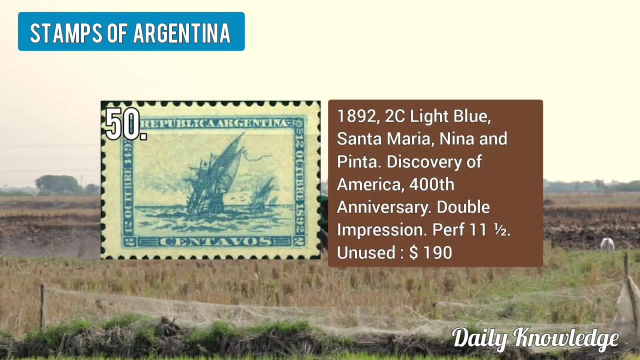 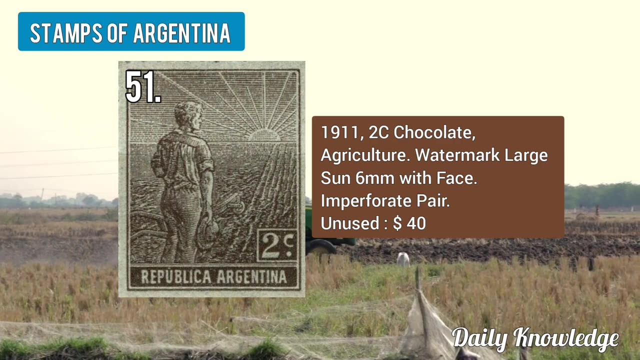 1867: 5C. Vermilion: groundwork of horizontal line Rivadavia stamp. 1892: 2C, Light Blue: Santa Maria, Nina and Penta. discovery of America. 400th anniversary 1911: 2C. Chocolate, agriculture workman. watermark- large sun, 6mm. with face. 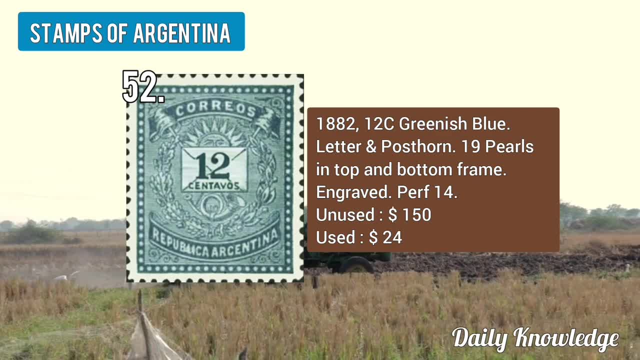 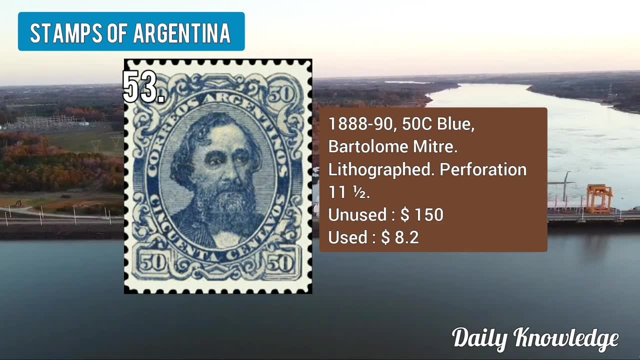 1882, 12C. Greenish Blue, later and post-war, 19 pulse in top and bottom frame. 1888-90, 1⁄2C. Blue bartholomew meter, lithographed and perforated, 11 1⁄2. 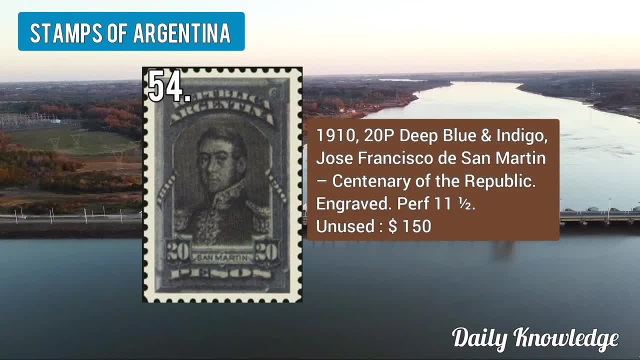 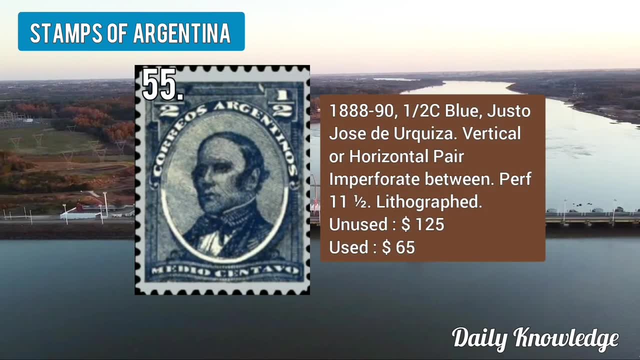 1910 20Pet Blue and Indigo Jaws Francisco D San Martin. Centenary of Republic 1888-90. 1⁄2C Blue Justo Jaws D Urquiza, vertical or horizontal pier, in-perforated. 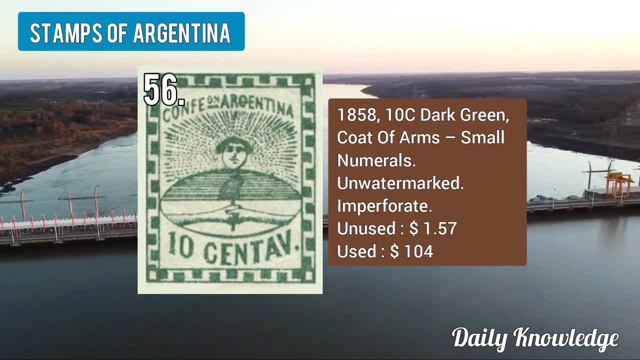 between 1858: 10C. Dark Green coat of arms: 1⁄2C. Blue bartholomew meter, lithographed and encoded. Euphrates: 16.5C. Silver, blue and rainbow: 6.3C. Red Denta, 10-1, 1898, after 10 years. 1891. 2.45P. Villagra, 1.65C. Greenish Black Peter by Michelangelo. 1891. 1⁄2C White, 2.45C Black. 5.5C Black, 4.1C Black, 4.2C Black, 4.1C Black. 1891: 1⁄2C. Black, 4.5C. Red, 5.8C. Black, 3.5C. Black, 3.5C, Red, 5.0C, White, 6.5C. Black- 2⁄2C. Black- 5.8C. Black- 5.6C. Greenish. Black- 5.8C. White- 5.8C. Black- 3.7C. Black- 5.9C Black- 5.2C Black- 7.7C Black. 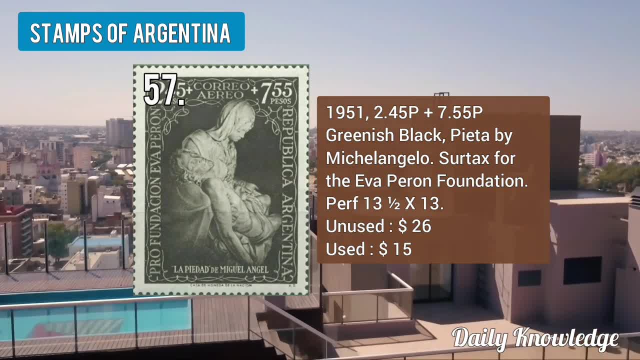 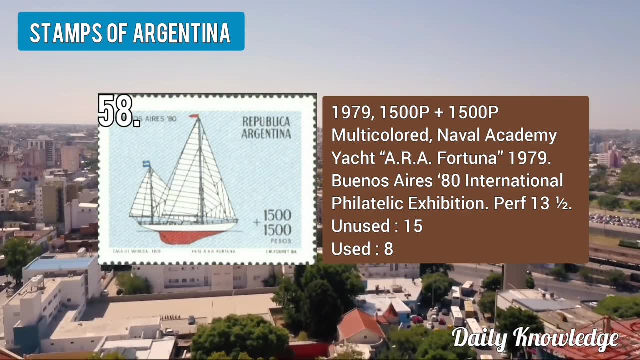 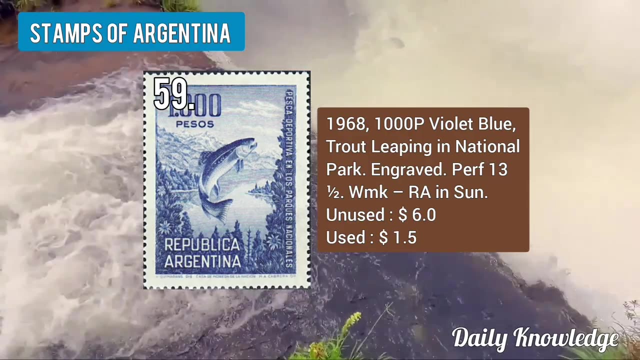 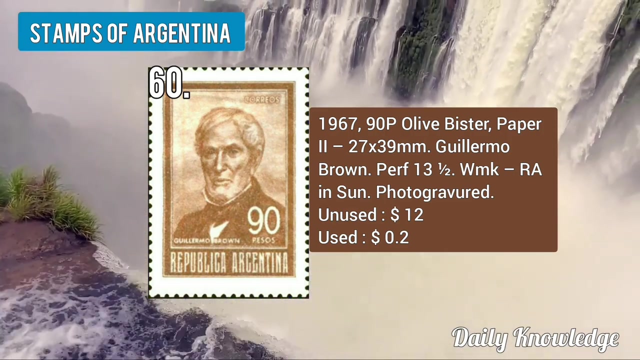 7.55P Greenish Black Peter by Michelangelo, Then 1979, 1500P plus 1500P Multicolour Naval Academy Jet 1968. 1000P Violet Blue Trout Leaping in National Park 1967. 90P Olive Pistachio Paper 2. 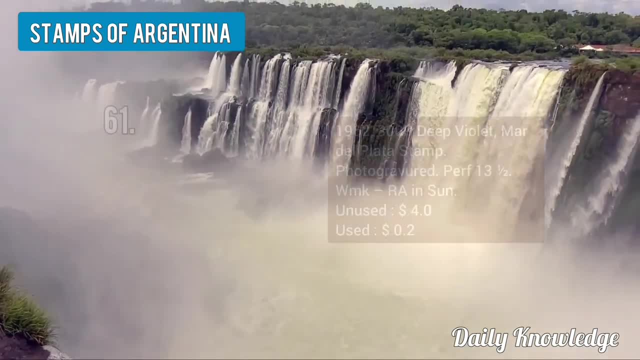 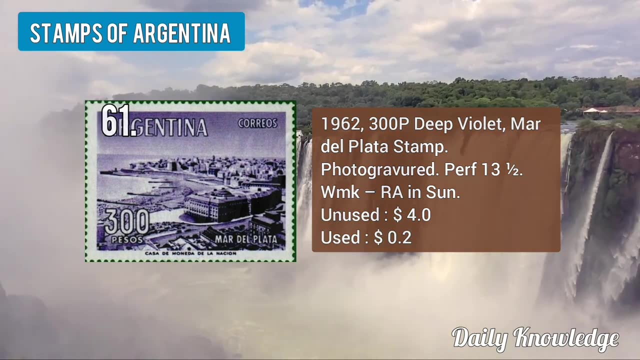 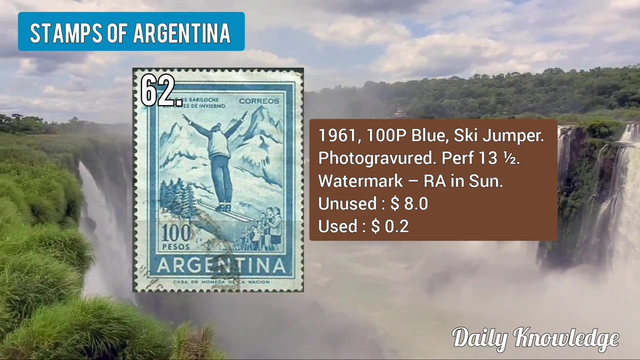 Killer Bow Brown, Perforated 13.5. Now this is 1962: 300P Deep Violet Martel Plata Stamp Photographer and Perforated 13.5. 1961, 100P Blue Skyjumper Photographer, Perforation 13.5. 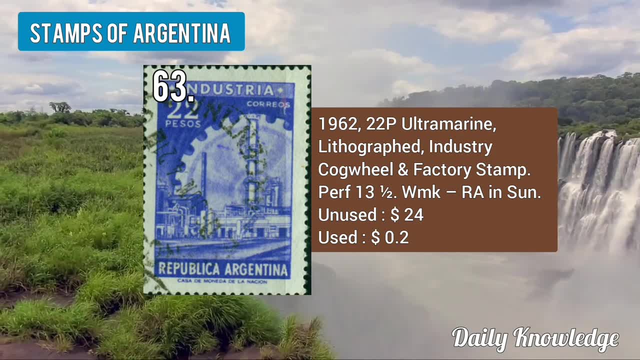 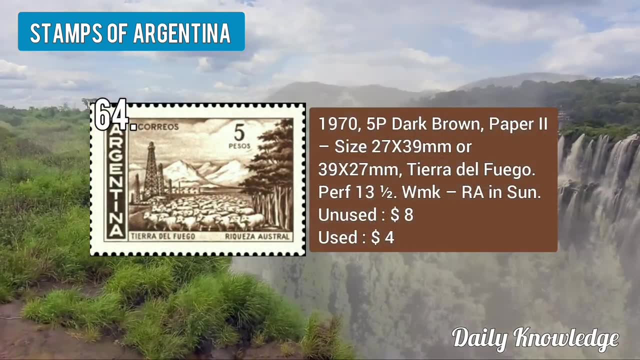 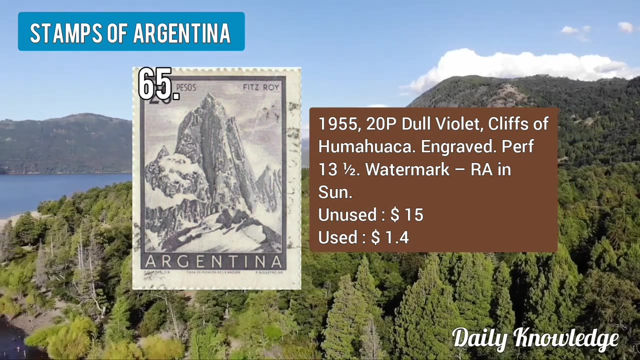 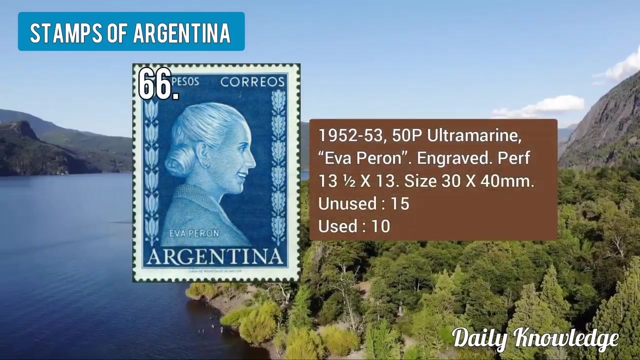 1962, 20P. Ultramarine Lithographed Industry Cocktail and Factory Stamp. 1970: Firebird Stem. 1955, 50P Dark Brown Paper 2, Tyra Del Fugo, Perforated 13.5. Now, 1955, 20P. Dull Violet Cliffs of Humahuaca, Engraved with Perforation 13.5. 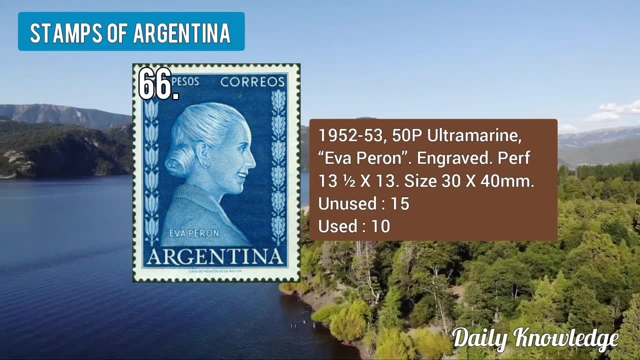 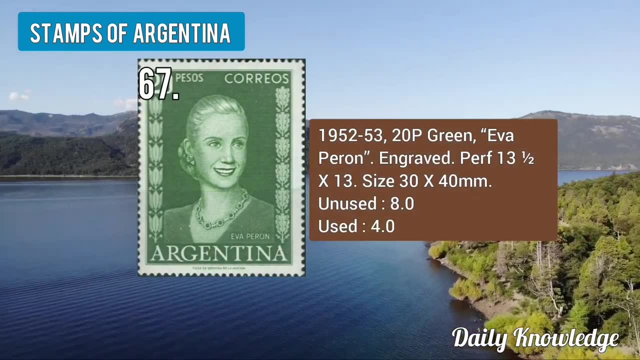 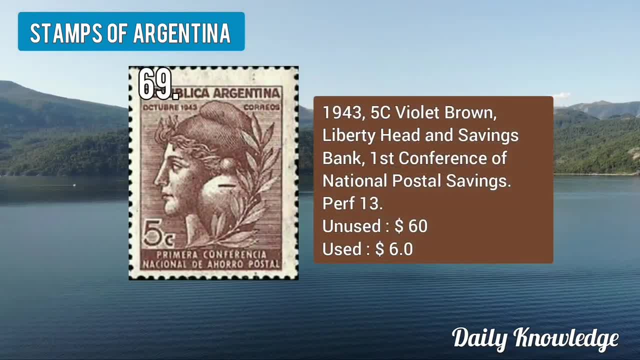 1952-53- 20P- Soprene Eva Perforated Stamp. 1952-53- 20P- Soprene Eva Perforated Stamp. 1952-53: 20P- Soprene Eva Perforated Stamp. 5C- Violet Brown, Liberty Head and Saving Bank. 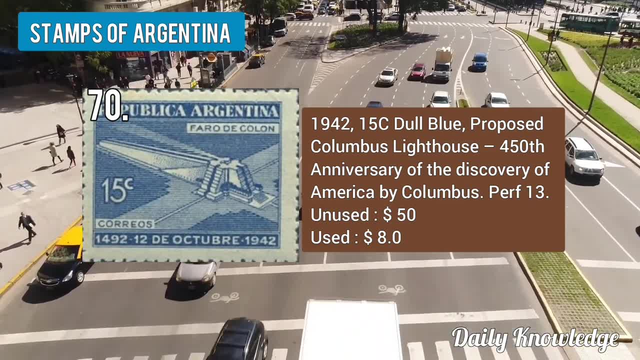 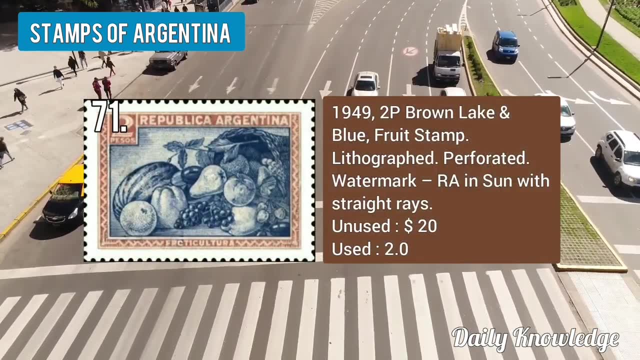 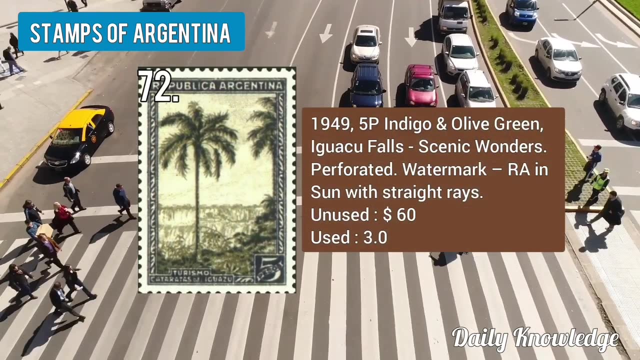 1942: 15C. Dull Blue, Proposed Columbus Lighthouse. 450th Anniversary of the Discovery of America by Columbus. 1949. 2P. Brown Lake and Blue Fruit Stamped, Dislithographed and Perforated. 1949, 5P. Integro and Olive Green. 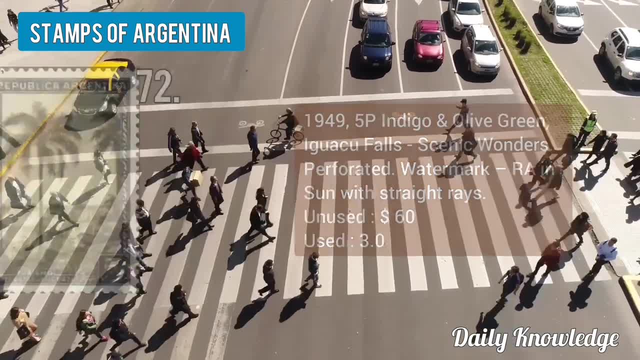 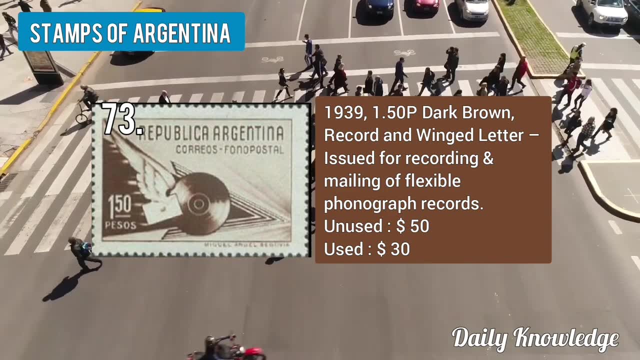 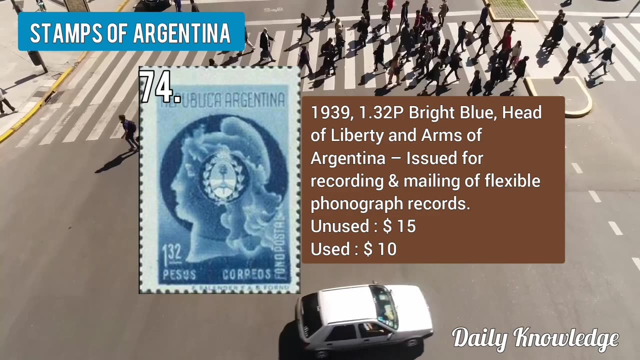 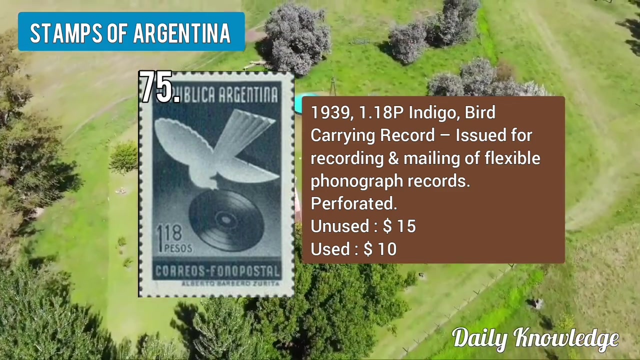 Iquacu Falls: Scenic Wonders. Perforated Stamp 1939. 1.50P. Dark Brown Record and Winged Ladder 1939. 1.32P. Bright Blue. Head of Liberty and Arms of Argentina 1939. 1.18P. Indigo Bird Carrying Record. 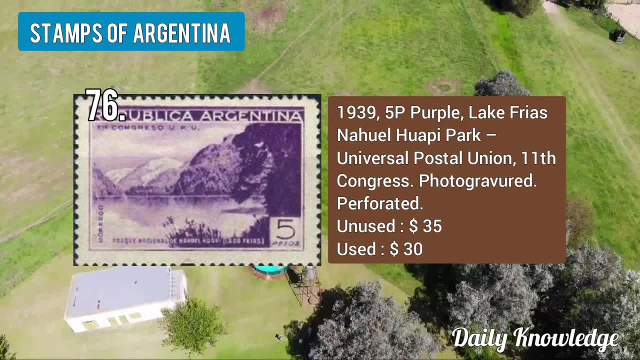 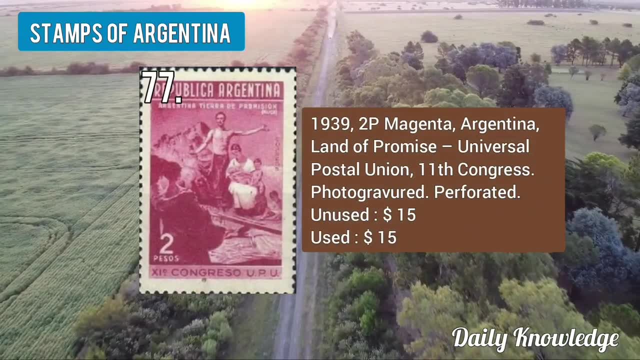 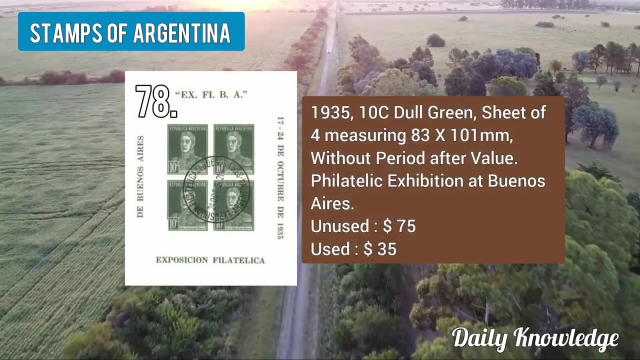 1939: 5P. Purple Lake, Frias. Universal Postal Union- 11th Conference 1939. 2P. Magenta, Argentina, Land of Promise, Universal Postal Union, 11th Congress 1935. 10C. Dull Green Sheet of Four, Without Period After Value. Philatelic Exhibition at Buenos Aires. 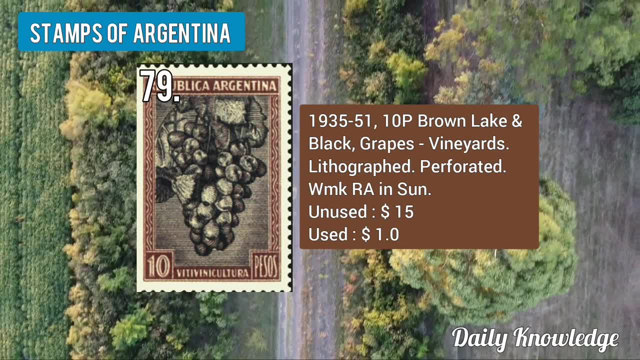 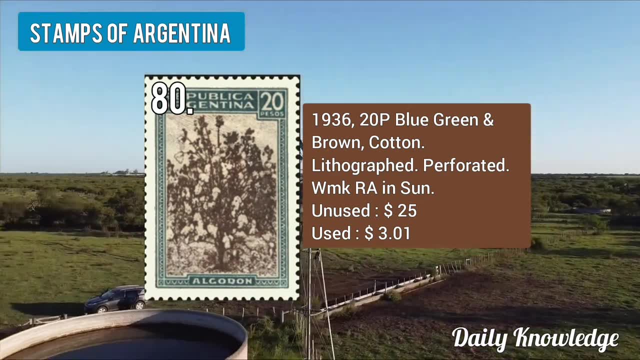 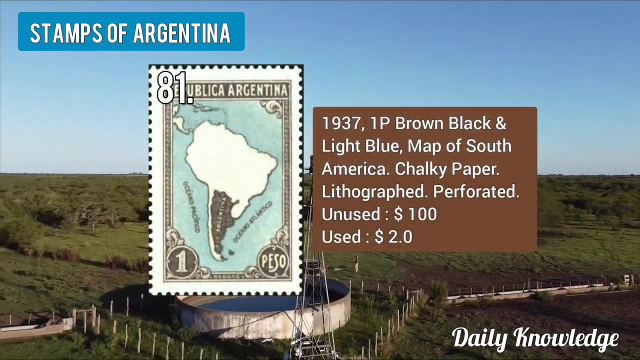 1935-51. 10P. Brown Lake and Black Grapes Wine Jards, Lithographed and Perforated 1936. 20P. Blue, Green, Brown Cotton Stamp, Lithographed and Perforated 1937. 1P. Brown, Black and Light Blue Map of South America. 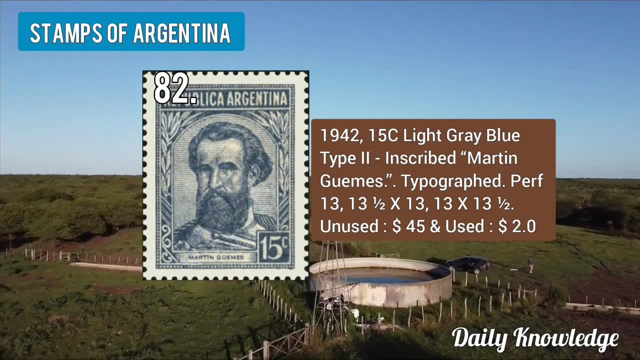 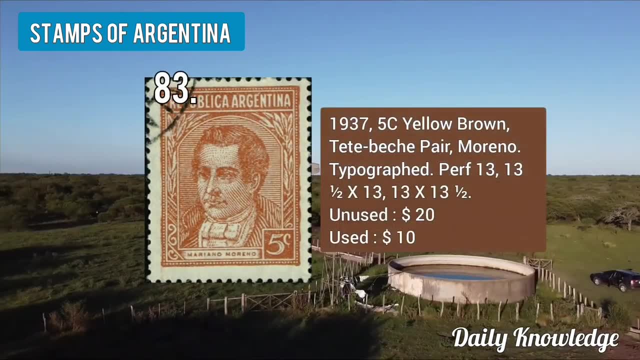 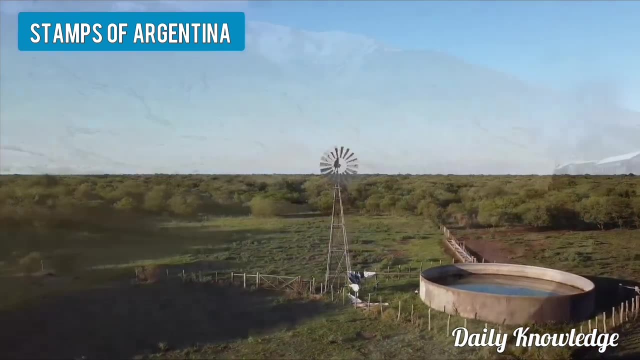 It is on chalky paper and it is lithographed: 1942-15C- Light Grey, Blue, Type II, Inscribed Martin Guiness. It is Typographed: 1937- 5C- Yellow, Brown, Tattooed Bear Moreno. Typographed and Perforated. 1937- 5C- Yellow, Brown, Tattooed Bear Moreno. Typographed and Perforated. 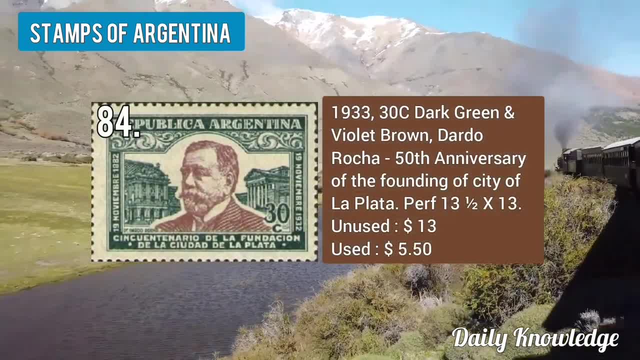 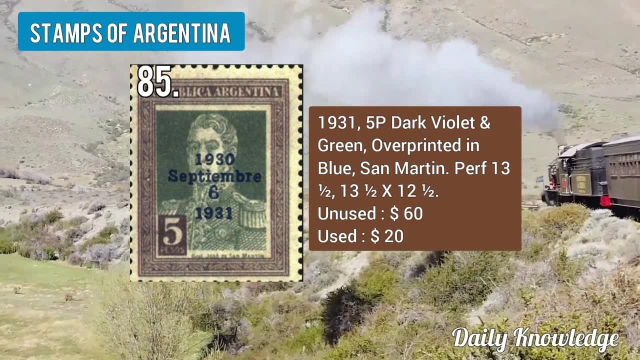 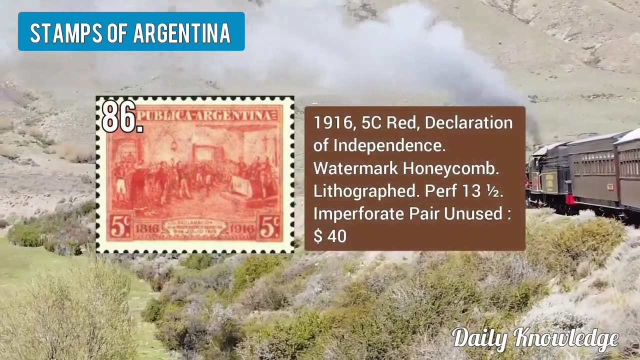 The 1933-36 Dark Green and Violet Brown. Dardo Rocha. 50th Anniversary of the Founding of City of La Plata, 1931. 5P. Dark, Violet and Green Overprinted in Blue. St Martin Stamp 1916. 5C. Red Declaration of Independence. Watermark: Honey Combed. 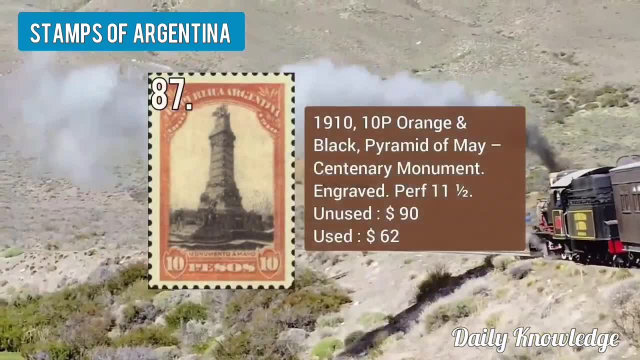 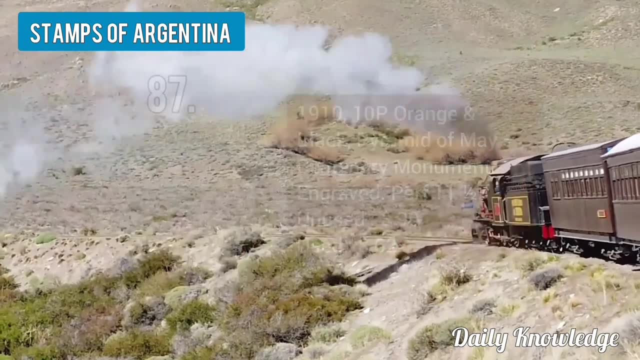 It is Lithographed and Perforated: 1910 10P. Orange and Black Pyramid of May Centenary- March Pyramid of May- Centenary Monument. It is Engraved and Perforated: 1902 5C. Deep Blue River- Port of Rosario.